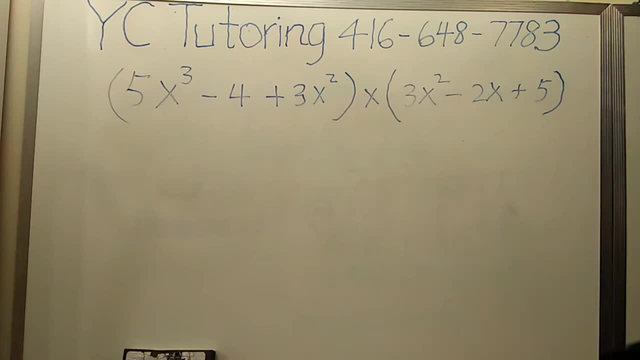 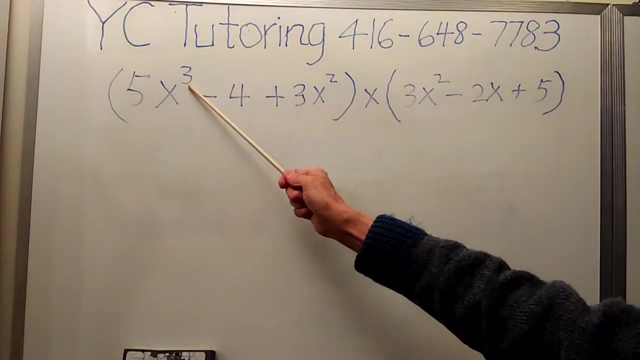 Okay, we multiply these two polynomials. First of all, we noticed that this is not in the right order. We noticed that this is not in the right order. You see cube here and square here. You see cube here and square here. 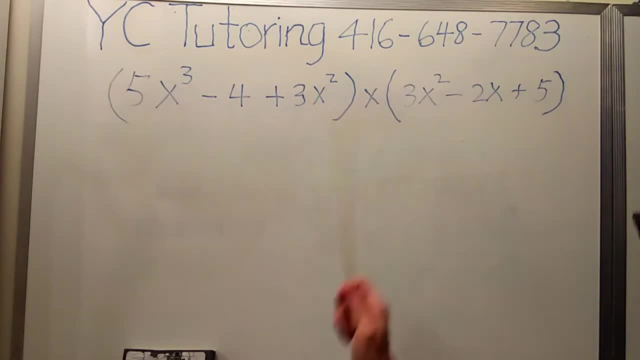 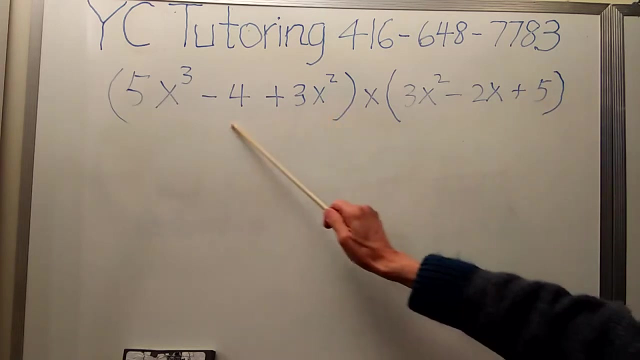 we should put this in the middle right, cube square, and so on. So let's rewrite this. This is okay, because you see, square and this is exponent 1, and this is a constant. So I need to rewrite this. 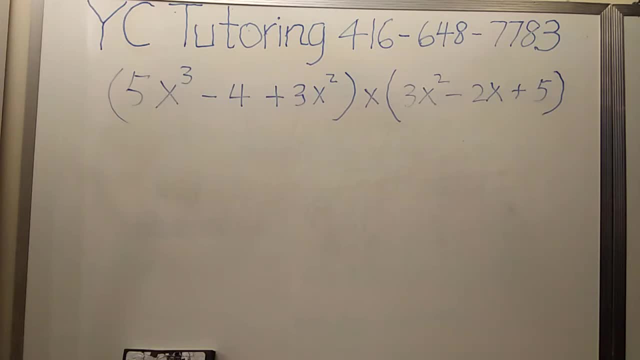 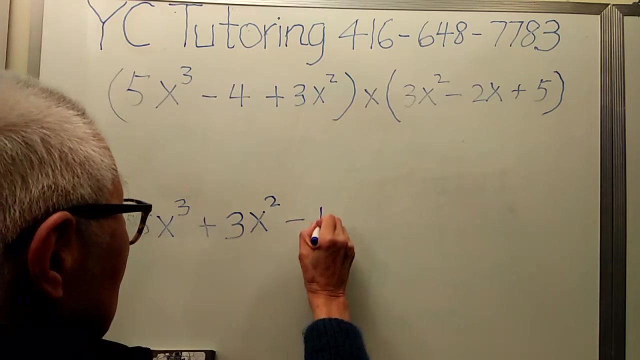 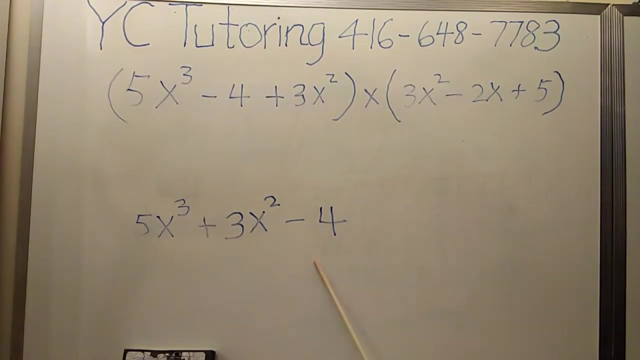 and then multiply. Okay, and then multiply. I have rewrite this. put this in the middle, put this in the second term: power 3,, power 2, and no x. power 3,, power 2, and no x. 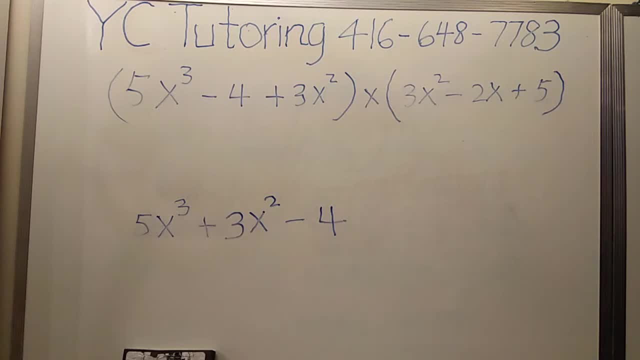 Before I do multiplication, I still need another term. I still need another term because I need 3,, 2, and 1,, because I need 3,, 2, and 1, and then constant. So what I write is: 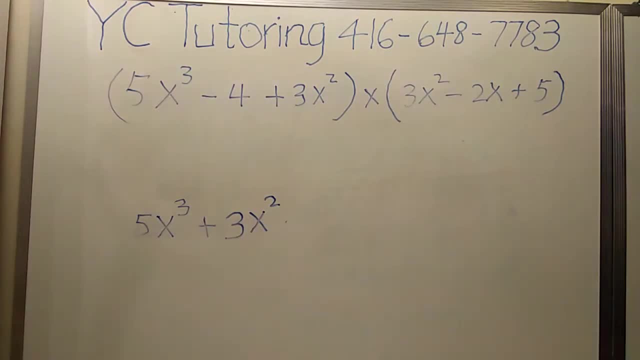 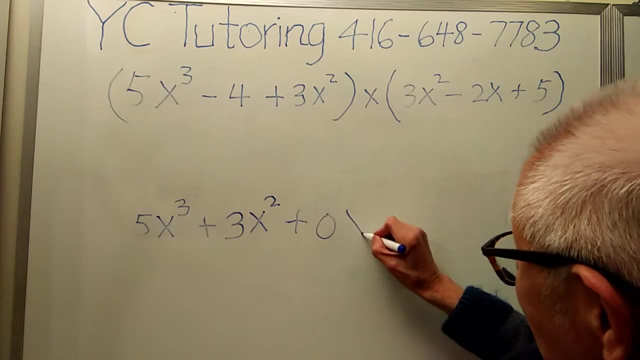 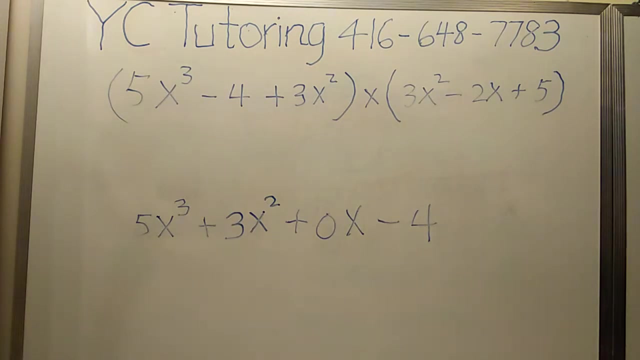 So what I write is. So what I write is plus 0 times x, plus 0 times x, plus 0 times x, and then minus 4.. and then minus 4.. Now I'm okay. Now I'm okay. 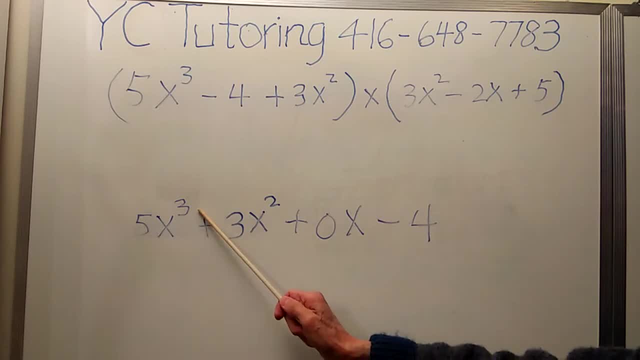 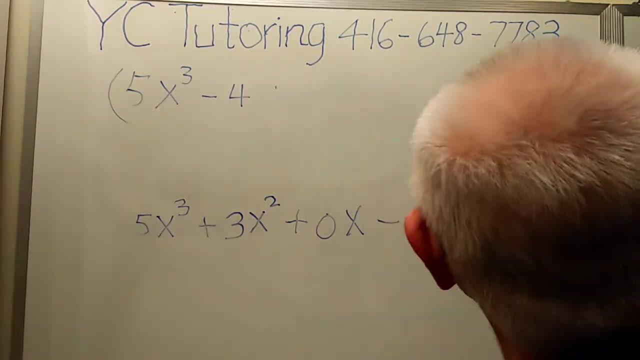 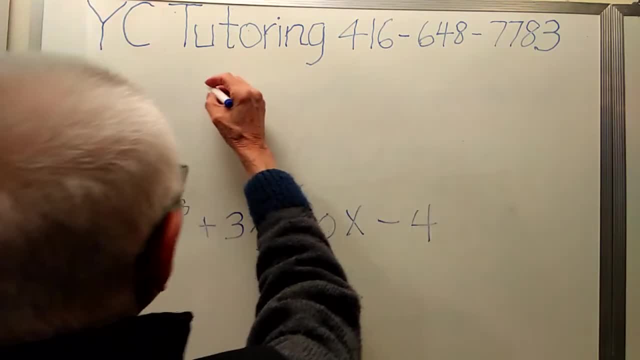 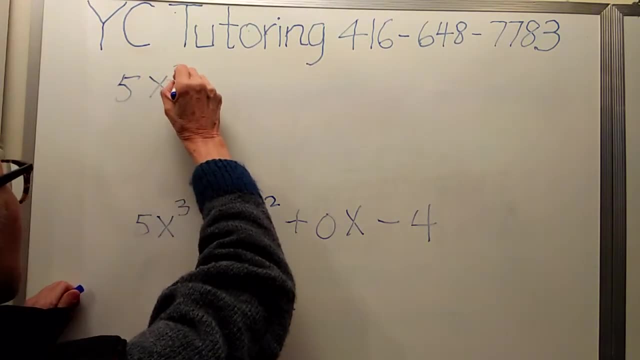 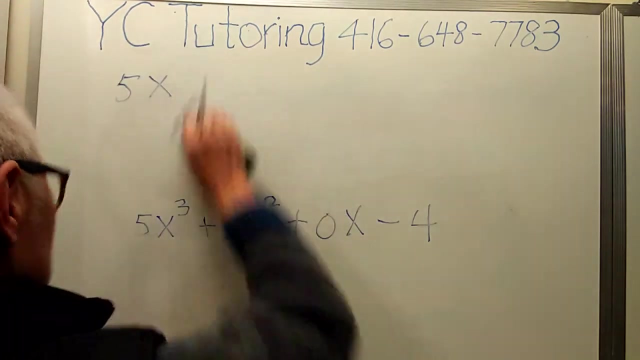 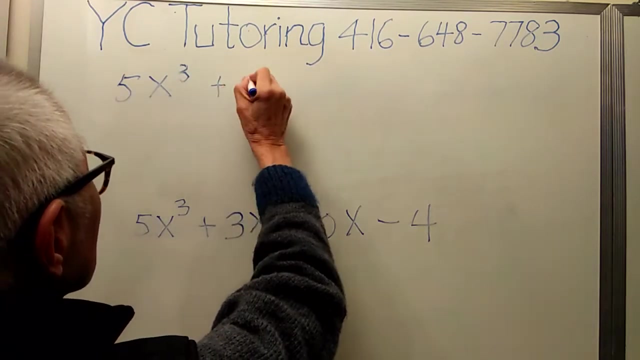 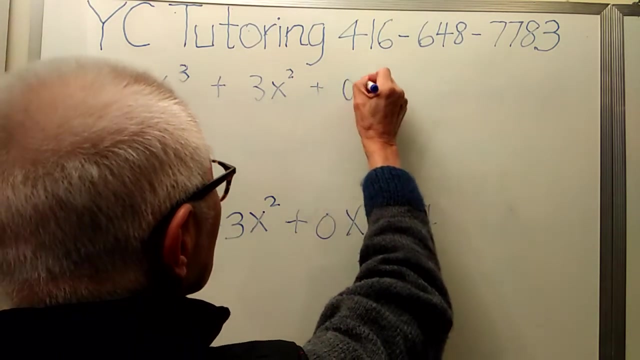 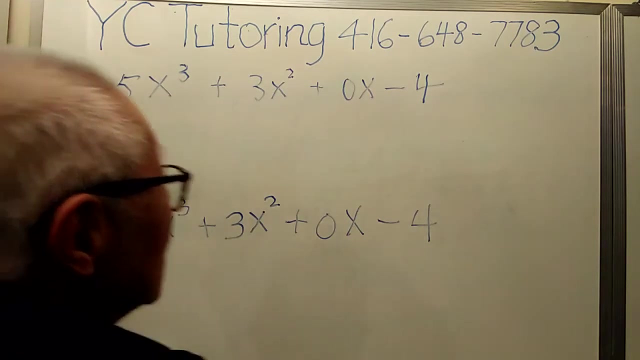 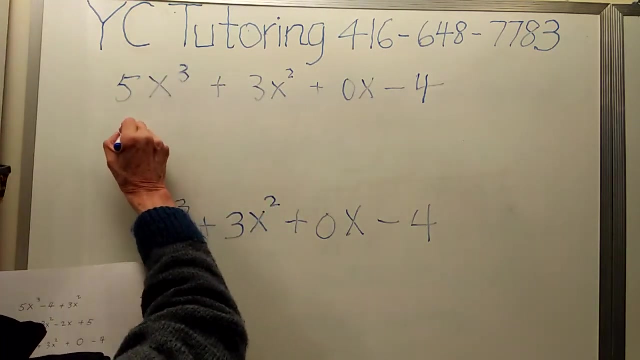 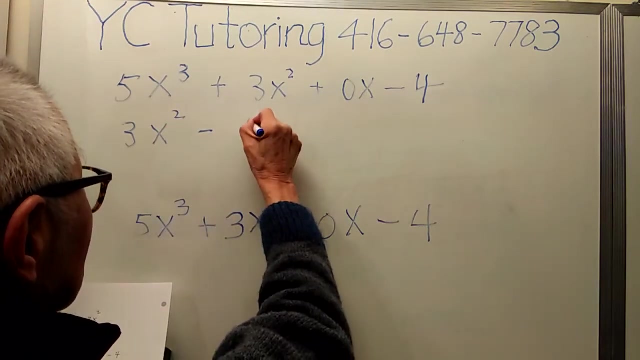 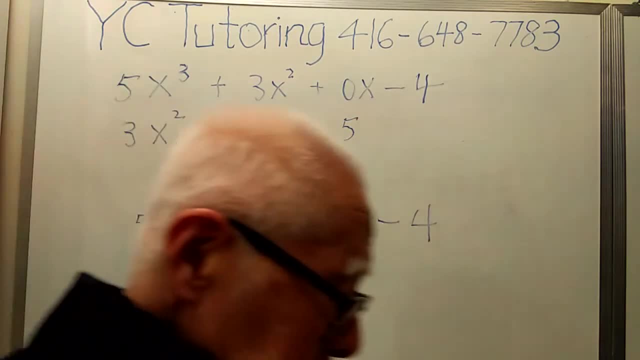 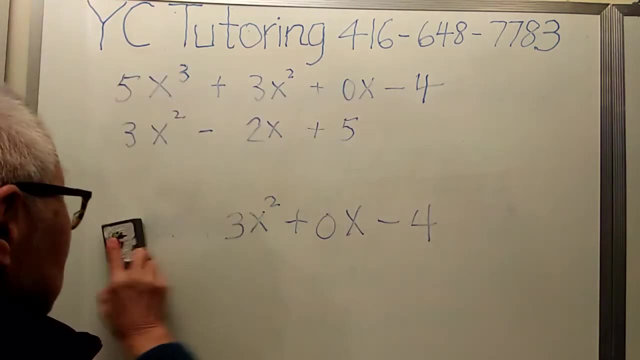 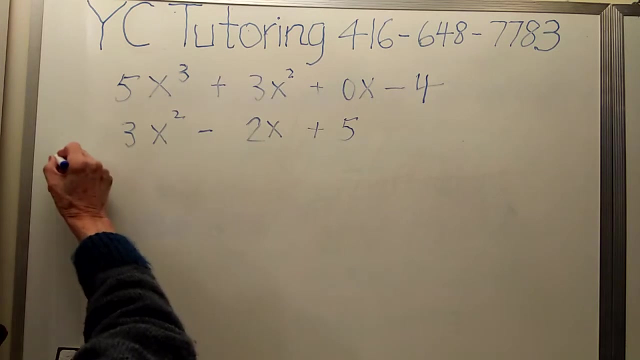 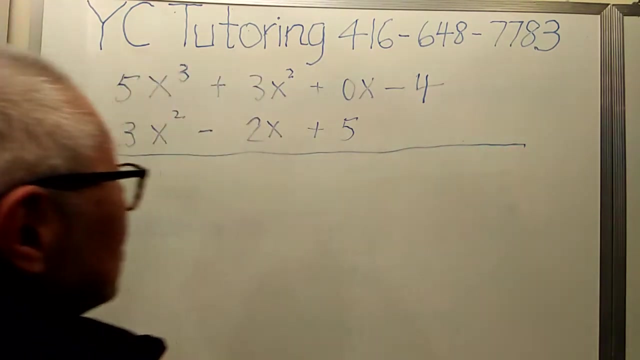 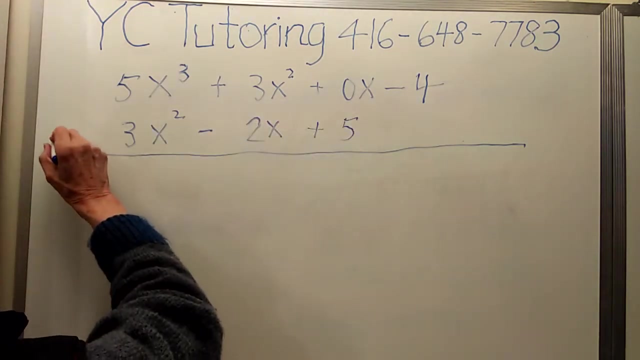 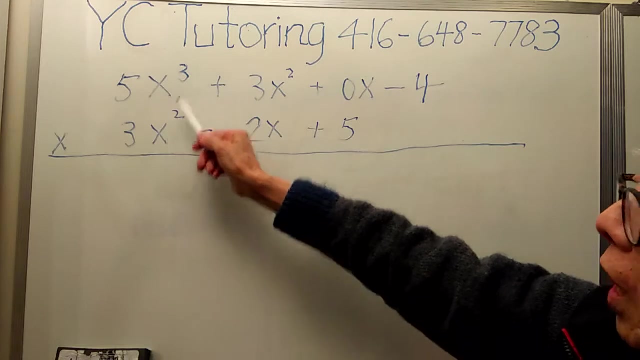 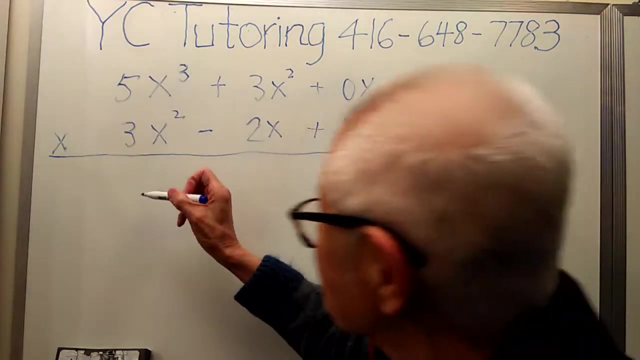 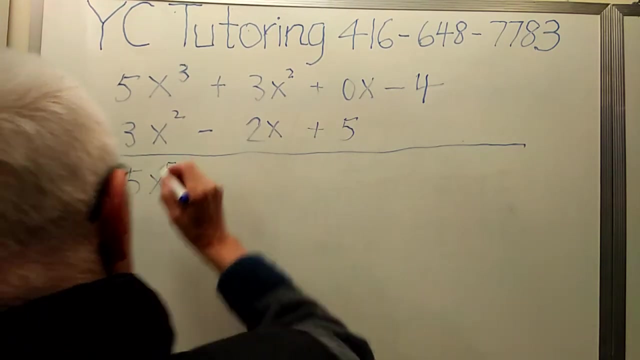 Okay, So I multiply this. So sorry that this pen doesn't work very well, But let's go on. So we multiply This times. that is 15x to the exponent 5.. And the next is this term: multiply this term. 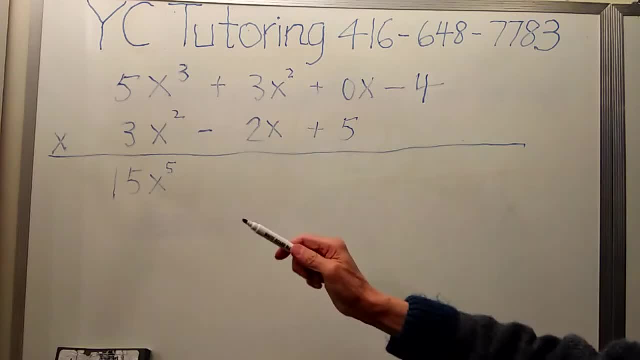 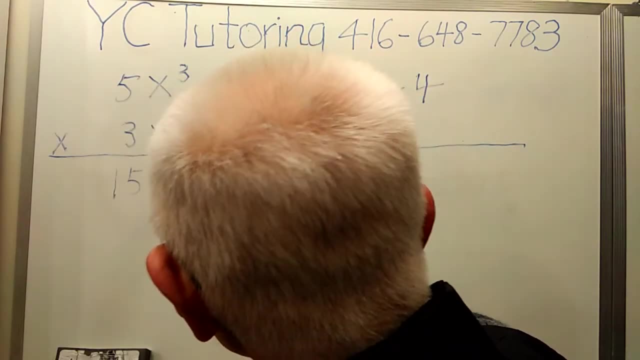 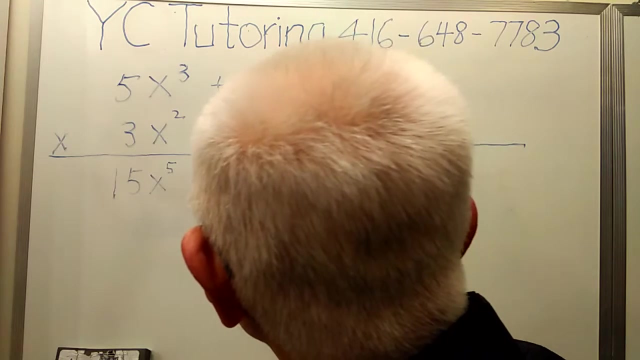 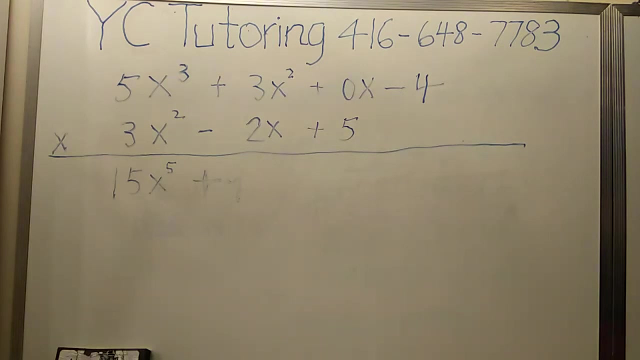 I have 9x squared minus 2x squared X to the exponent 4.. Oh my, I cannot write this Such a poor quality pen. Oh, Let's see, I may have another one, but it's not this color. 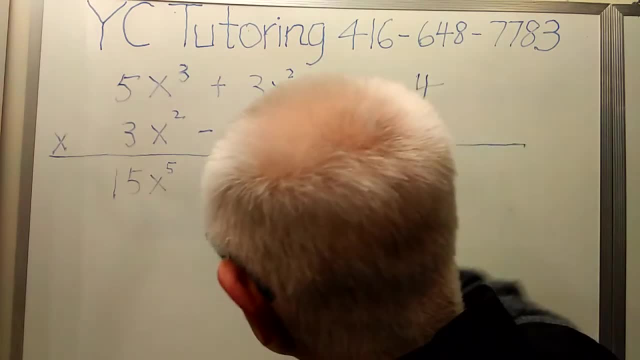 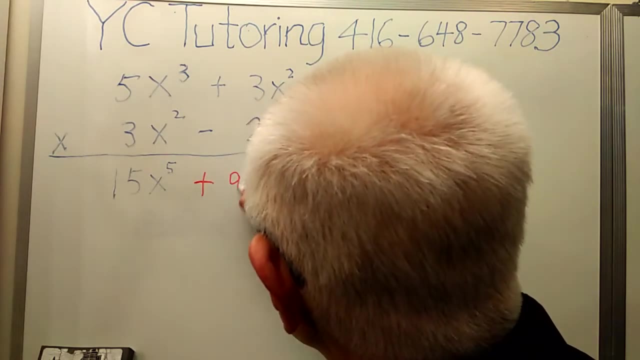 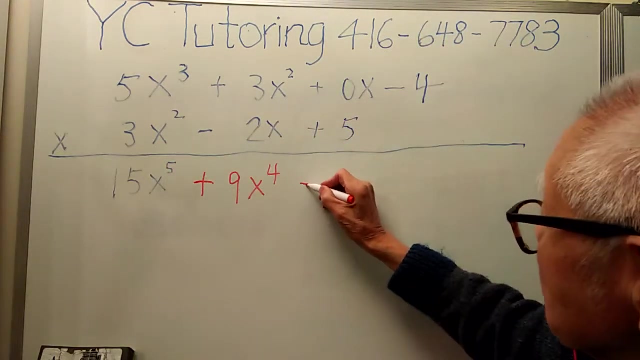 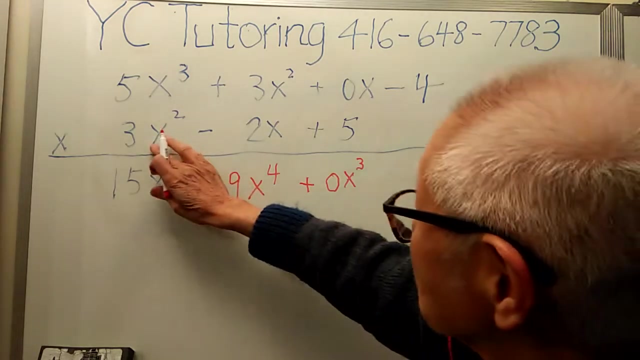 Let's see Whether you can bear with me. I have to use another pen. 9x to the power. 9x to the power 4. This times that is 0.. 0x to the power 3. This times that is negative 12.. 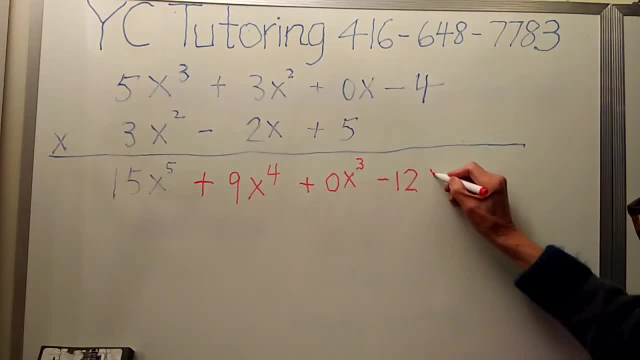 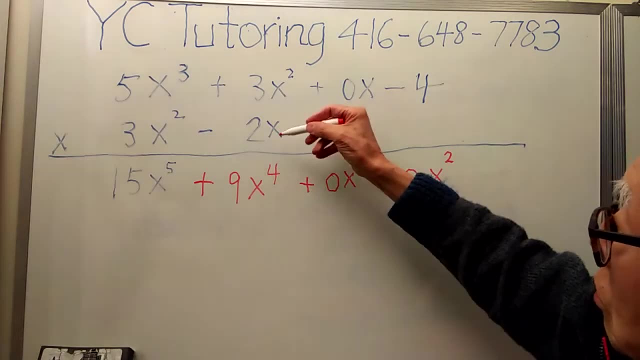 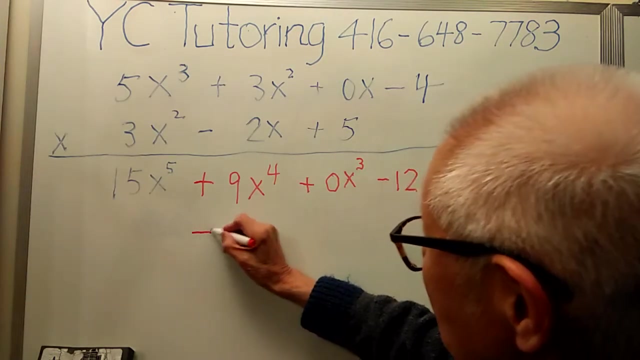 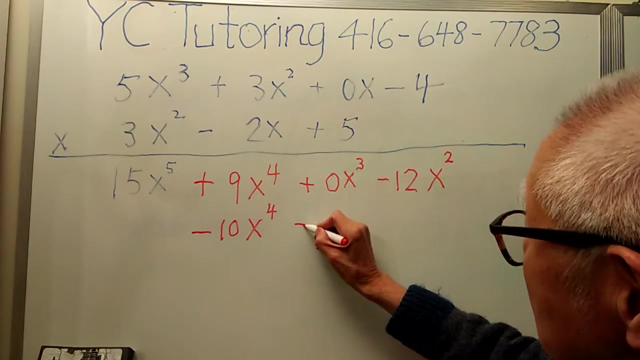 It's negative 12.. Negative 12x squared. Okay. The next is: this times that, which gives me negative 10x to the power 4.. Negative 10x to the power 4.. And this times that is negative 6 to the power 3.. 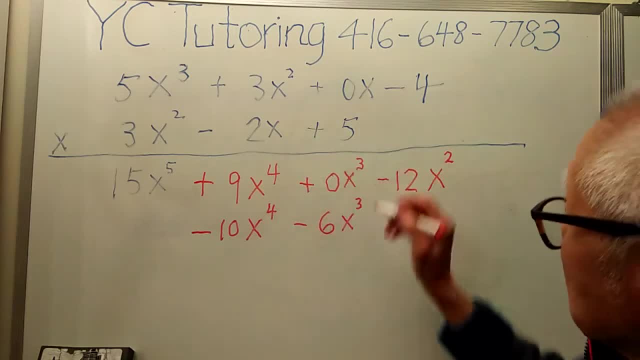 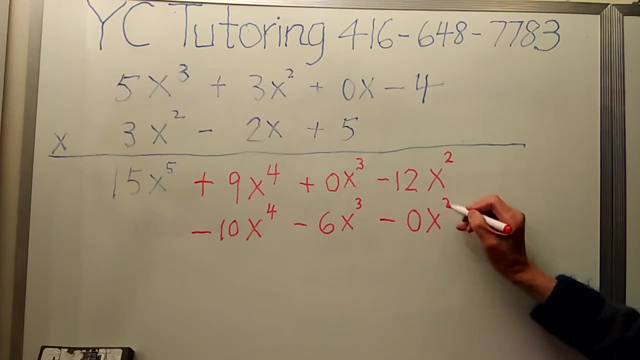 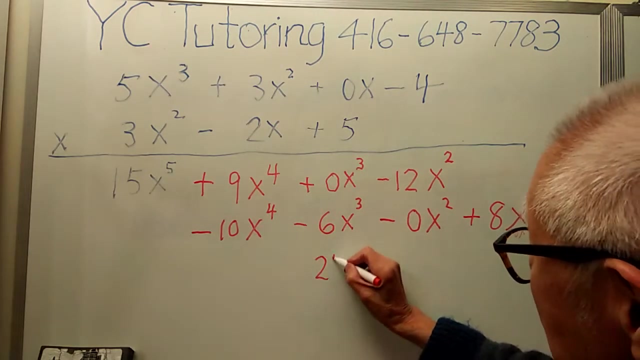 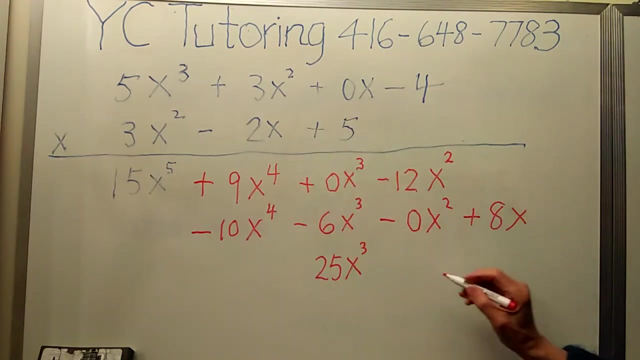 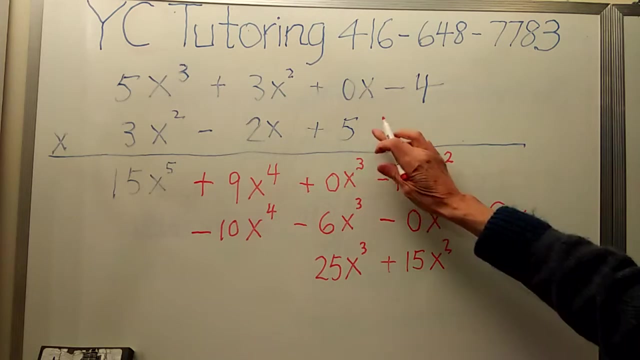 Remember 4x, And this times that is 0.. This times that is negative, negative becomes positive, which is positive: 8x. Okay, the next is: this times that is 25x cubed. This times that is 15x squared. 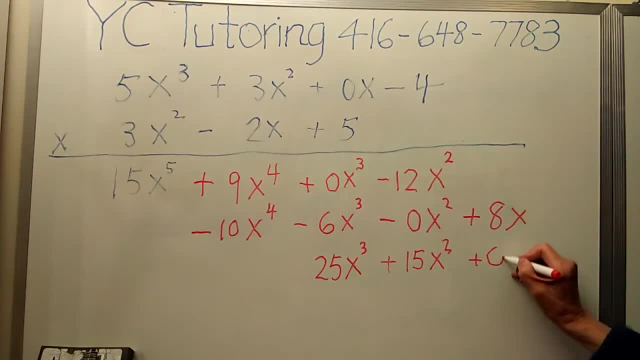 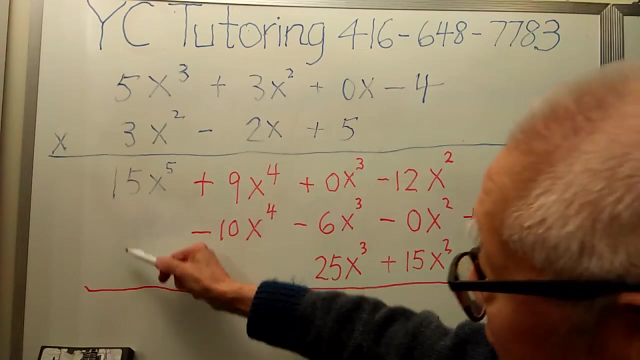 This times that is 0x. Okay, This times that is minus 20.. Okay then, just like usual multiplication, we need to add everything. Okay, this is: add So 15x to the exponent 5, adding nothing here, nothing here. 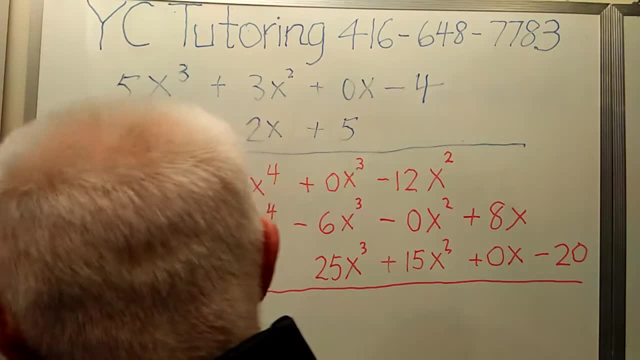 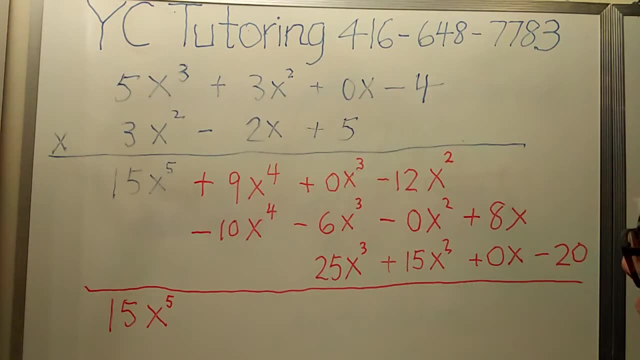 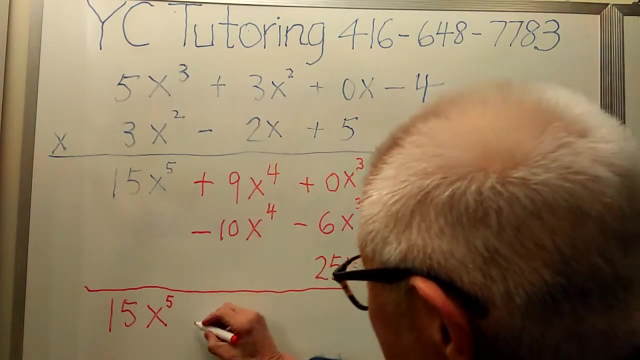 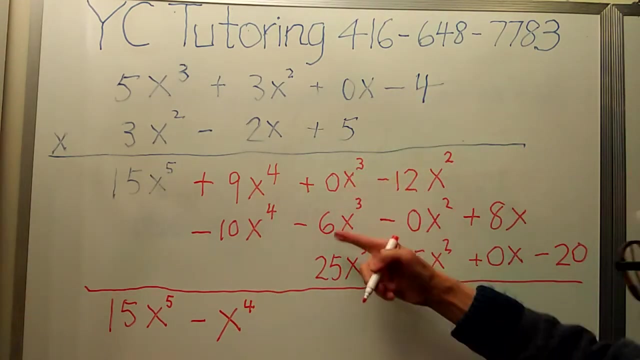 So it's Okay. It's 15x to the power, 15x exponent 5.. This and this put together is add together is negative x exponent 4.. The three times this is 0. So you just add these two times, which is plus. 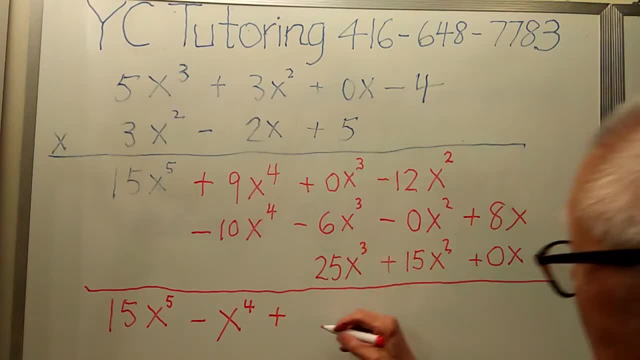 Okay, Okay, Okay, X cubed. Now, this is 0.. So you'll just put these two together. It should be plus five, Ah, plus three x squared. Well, this is square. This is squared. This is zero. 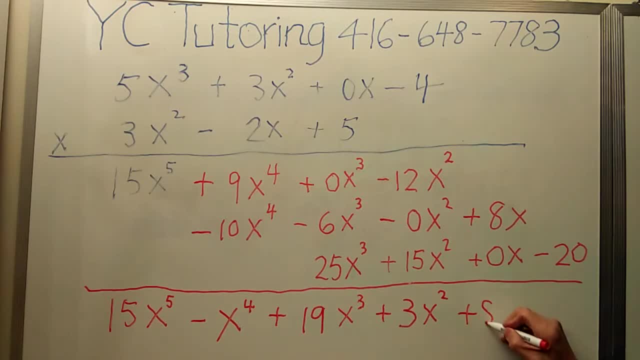 So it's 8x. Okay, This is minus 20.. So I have my results. This is the product. This is the result of multiplying two polynomials. This is how you do it. You follow me. I hope you follow everything right. It's not difficult. However, I want to introduce: 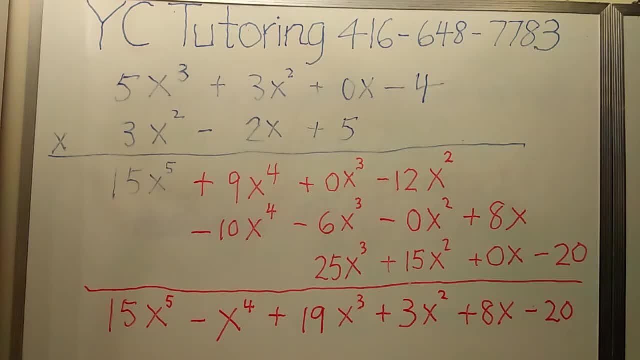 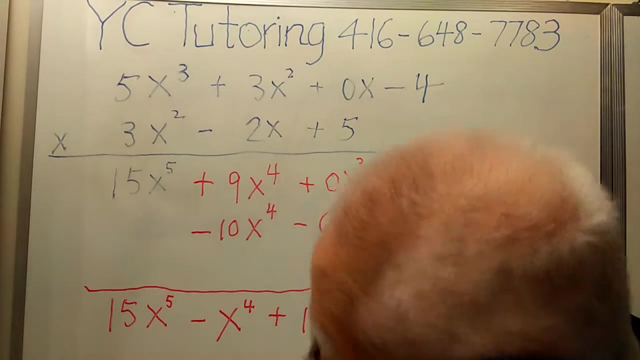 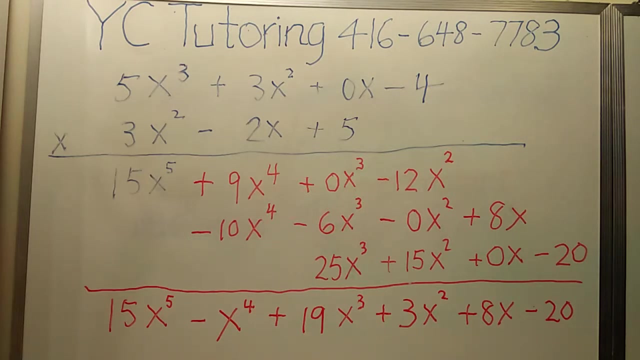 a method of detached coefficients. What does that mean? I separate the coefficients from the variables. This is how I do it. I just erase the X, All the X's. I need to erase it. I don't need it, because this is: if you write the X here, X there, it is just a. 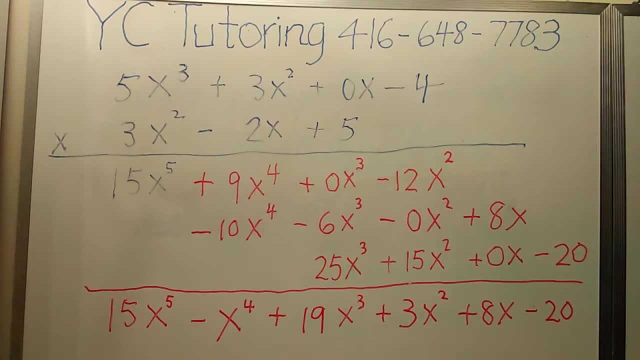 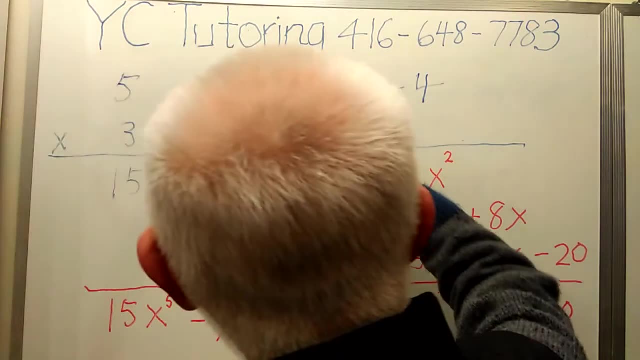 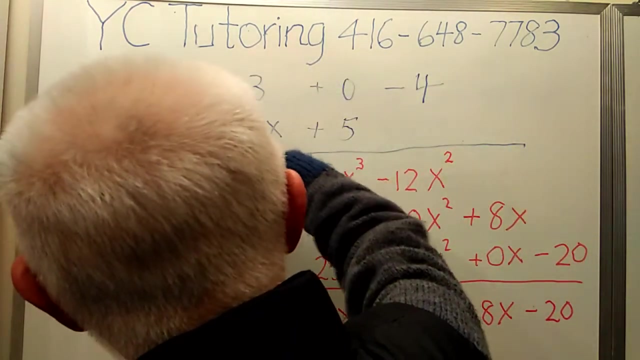 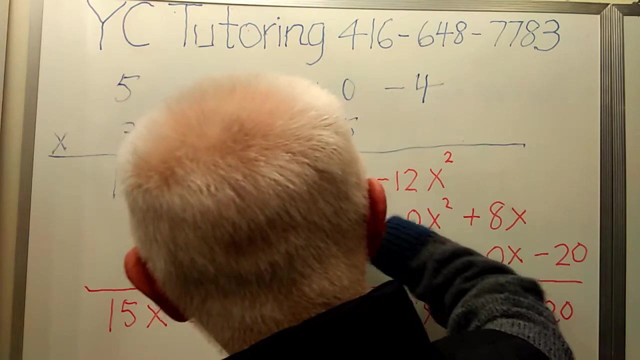 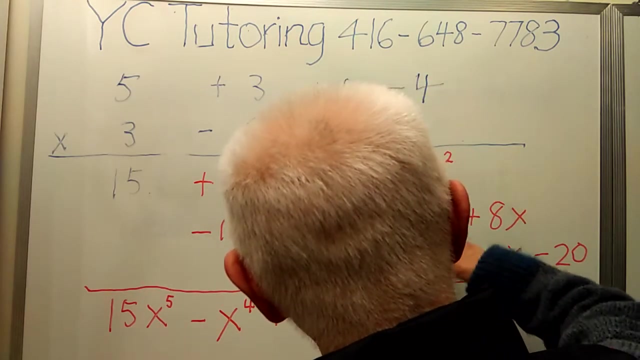 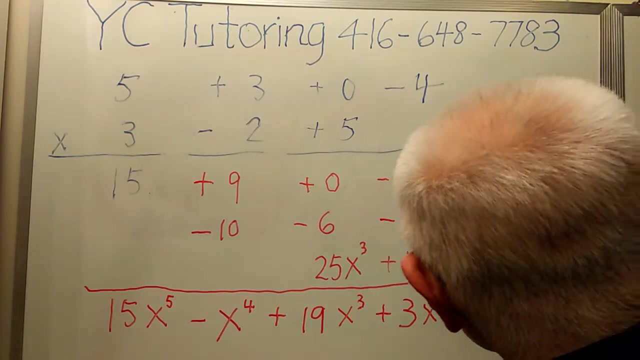 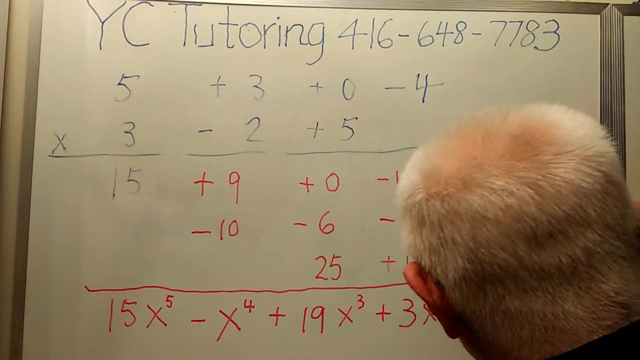 waste of time. Why do we need to write X? Let's erase it. Erase all the variables, all the unknowns, X, Okay. Erase all the variables at x, okay. Why do you want to erase? Erase all the variables. 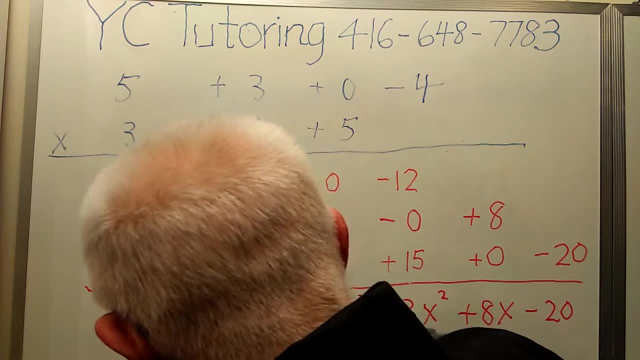 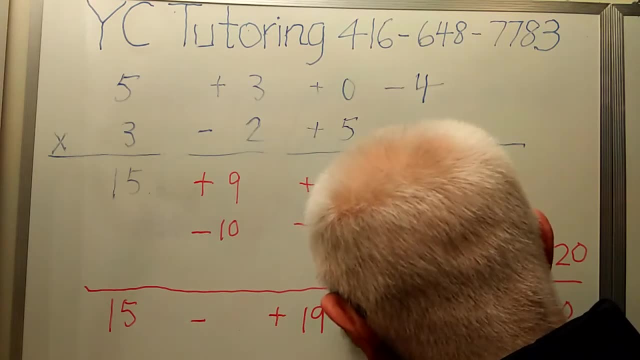 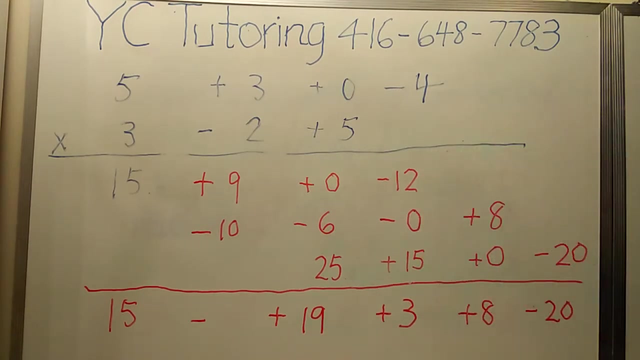 Erase Q, Erase Y, Erase X, Erase X. You see that if I want to multiply two polynomials, I just write down the coefficients of the first polynomial and the coefficients of the second polynomial, Then I just multiply this. 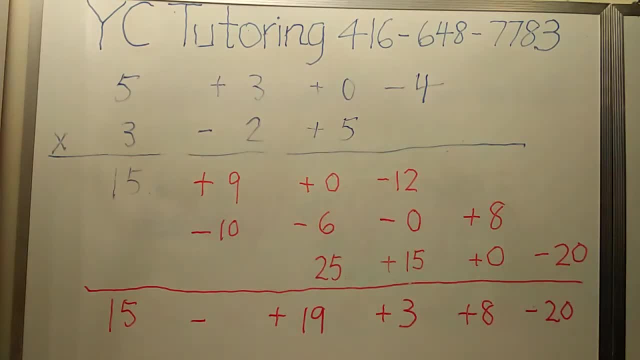 times that, this times that, and put down the results And multiply the usual way, but do not write x, Multiply and then, of course, this is multiplication. you need to add. Okay, so this is the result of adding, But what is my final result? The final result, of course, contains x.